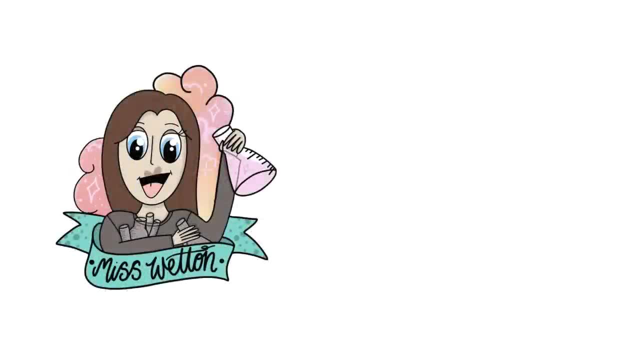 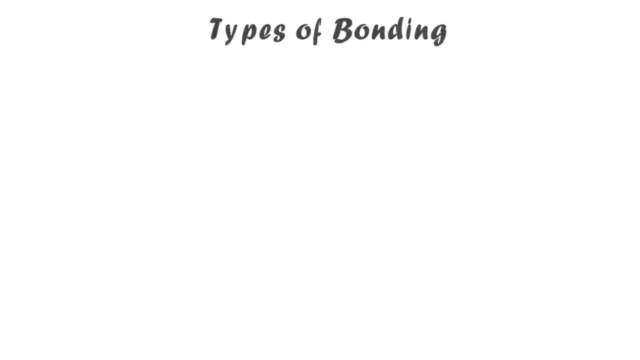 Hello, in this video we're going to look at the three main types of bonding that you'll see in Elements and Compounds and we're going to look at how each type of bonding occurs. The three main types of bonding are covalent bonding, ionic bonding and metallic bonding. 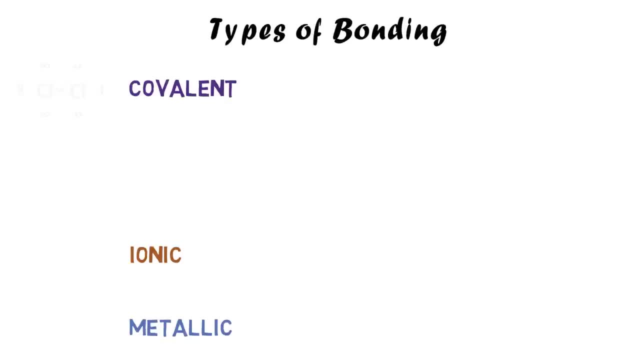 Covalent bonding occurs when atoms share electrons, so their outer shells overlap and they will share a pair of electrons. This only happens in non-metals, so metals are never involved in covalent bonding. There are two types of covalent bonding: Simple covalent. 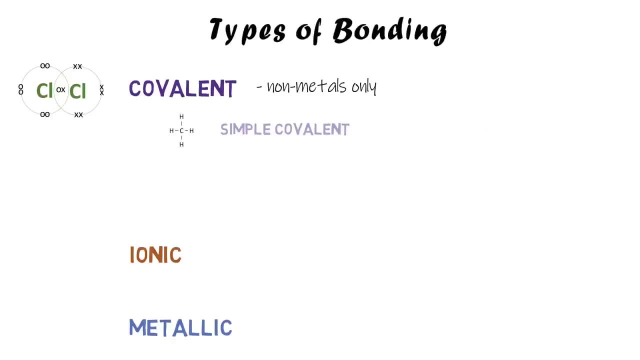 which is small molecules like CH4, H2O, CO2, with just a few atoms in them, and this makes up most of the covalent compounds. so almost all covalent compounds are simple covalent. There are a few exceptions which are giant covalent compounds Instead of small molecules. 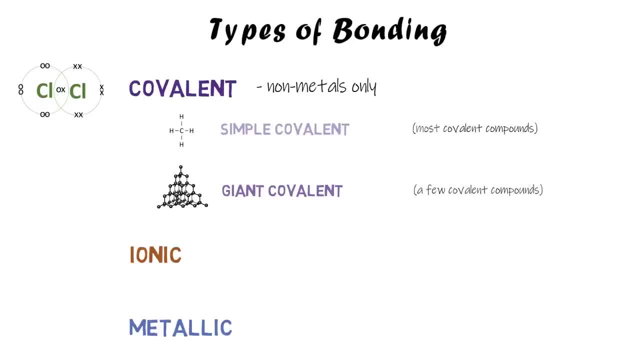 these have thousands of atoms joined together. They're still covalently bonded, but there are just a few of these examples that you need to know that form giant structures. Ionic bonding is not sharing electrons, it's giving and taking electrons. This happens when. 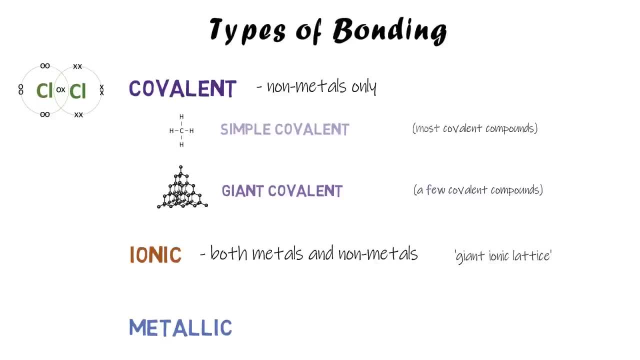 you've got both metals and non-metals together, You must have at least one metal and at least one non-metal. And when you've got both non-metals and non-metals together, you must have at least one electron. When they react together, they form this giant ionic lattice of positive and negative. 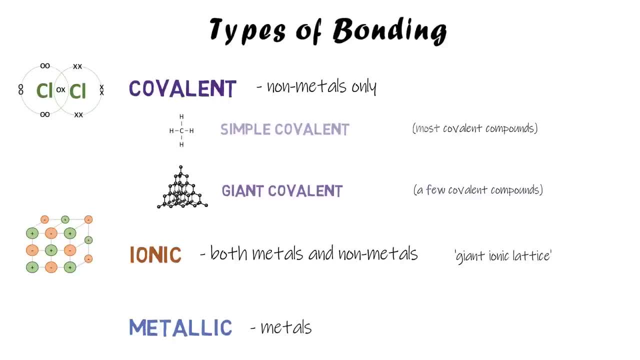 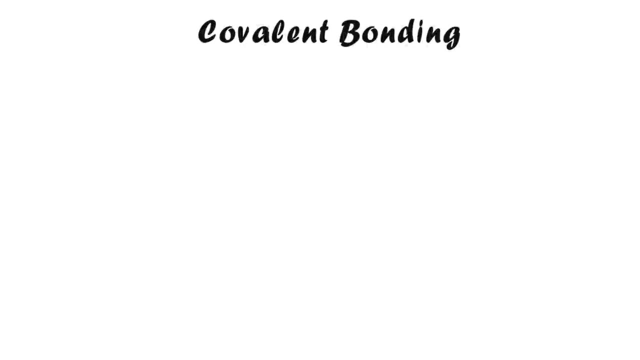 ions. And finally, metallic bonding occurs only within metals, so non-metals are never involved. We've got the positive ions and the delocalised electrons, So we'll start looking at covalent bonding. Covalent bonding happens only in non-metals. 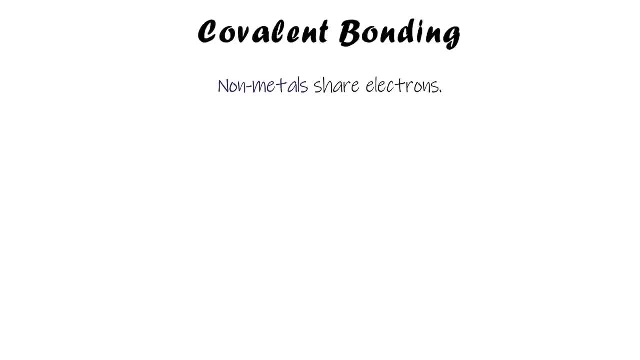 so we never have metals involved covalent bond in, and it happens when two non-metal atoms, or more than two, share a pair of electrons. so here we've got two chlorine atoms. their outer shells are overlapping and they are sharing a pair of electrons. this shared pair of electrons is a covalent bond and it joins the two atoms together. 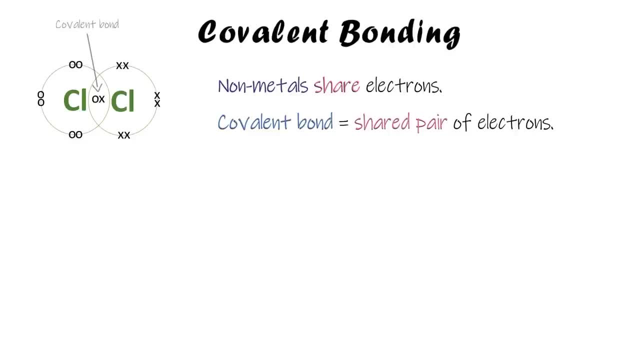 it's a very strong bond and it holds them together. so this xo in the middle is a shared pair of electrons and that is the covalent bond between the two atoms. this is a simple covalent molecule. we have the simple covalent and we also have giant covalent. simple covalent molecules are 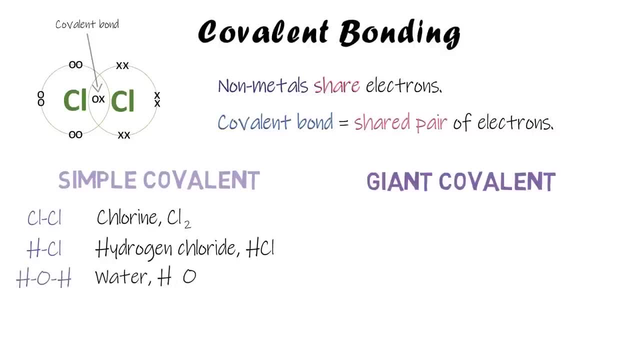 things like chlorine, Cl2, hydrogen chloride or hydrochloric acid, water, oxygen and carbon dioxide. so you can see, these are all elements or compounds that contain one, two, three, maybe four atoms, but anyway it's only a few. so when you've done that, you're going to want to make sure that you've. 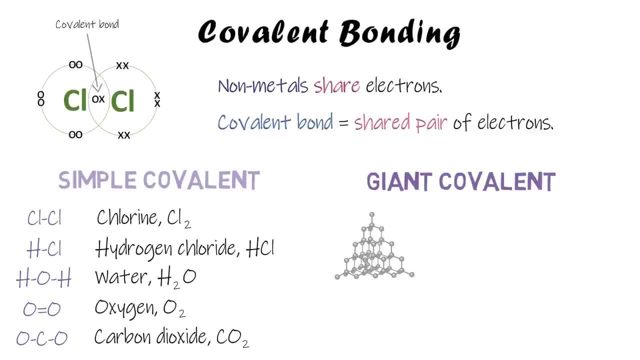 just got a few atoms in a molecule. that's a simple covalent molecule. giant covalent, on the other hand, is when you've got many thousands of atoms joined together. three examples of this would be the allotropes of carbon, diamond, graphite and graphene. instead of just three or four carbon atoms, you've 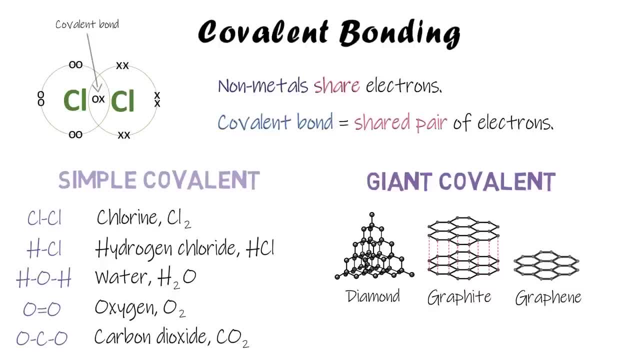 got hundreds or even thousands of atoms joined together in a giant structure. the one other example of this you need to know is silicon dioxide. you just need to remember these four examples. so you need to remember these four examples. so you need to remember these four examples. so 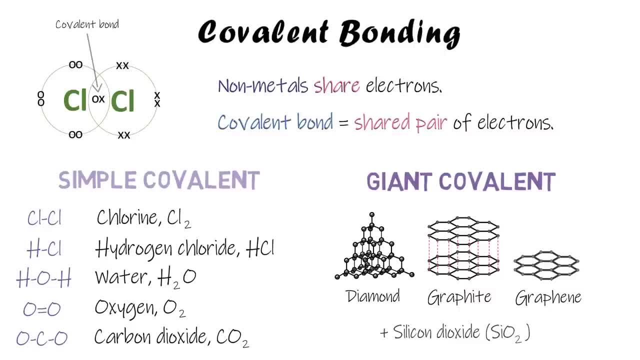 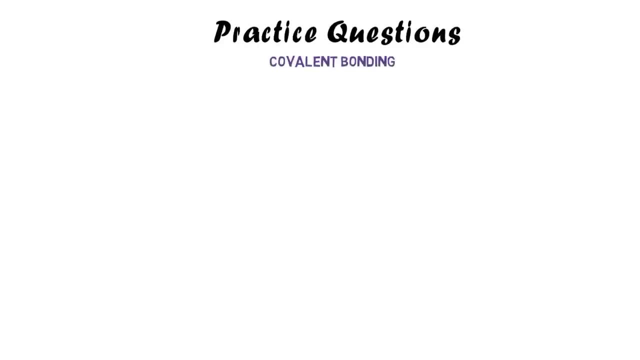 if it's covalent. if it's not one of those four examples, you can assume that it's a simple corvette compound. here is some practice questions for covalent bonding. number one: what is a covalent bond? number two: which types of elements form covalent bonds? and number three: which of these compounds has a? 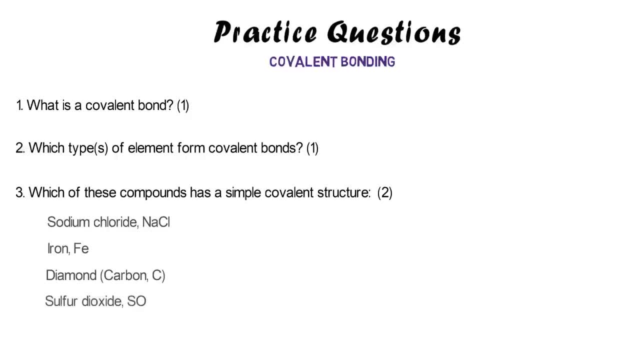 simple covalent structure. we've got sodium, chloride, iron, diamond, sulphur dioxide and oxygen. pause the video and have a go at these questions. A covalent bond is just a shared pair of electrons. It's a pair of electrons that are shared between two atoms when their outer shells overlap, as shown. 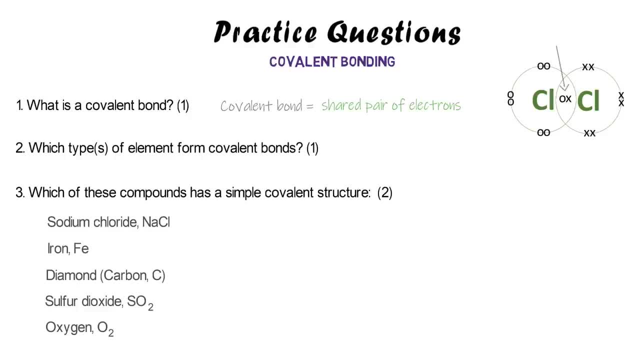 in this diagram. So in this diagram it's the XO pair in the centre of the two atoms. That is your covalent bond. Covalent bonding can only occur between elements that are non-metals- either two atoms of the same element or it can be different elements. They have to be non-metals, And of that. 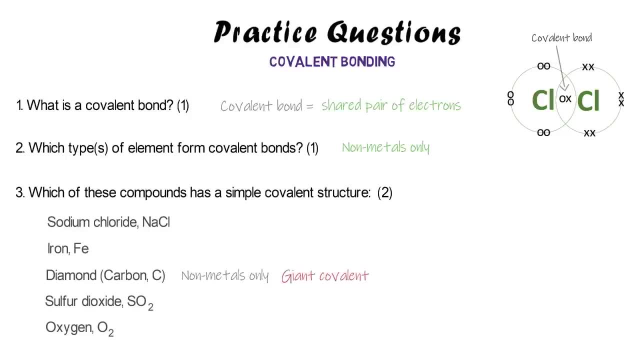 list. the only ones that are made of non-metals only are the last three, But diamond is one of those examples where it's a giant covalent, whereas sulphur dioxide only has three atoms and it's covalent. So that's going to be simple covalent. 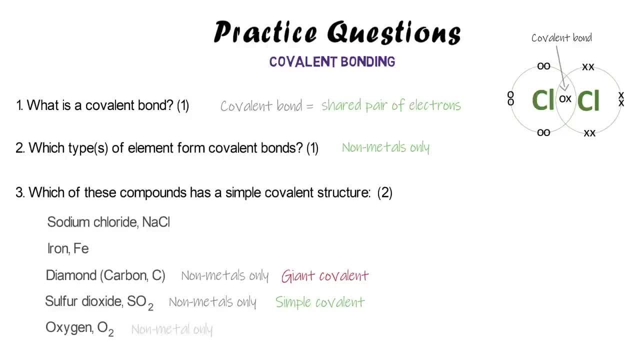 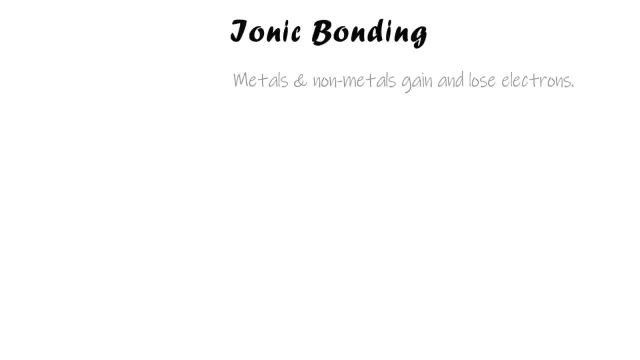 And then oxygen- O2, again we know it's covalent because oxygen is a non-metal And because there are only two atoms in that molecule, it's going to be a simple covalent. Now we're going to look at ionic bonding, which is a little bit different to covalent bonding. This happens when you've got 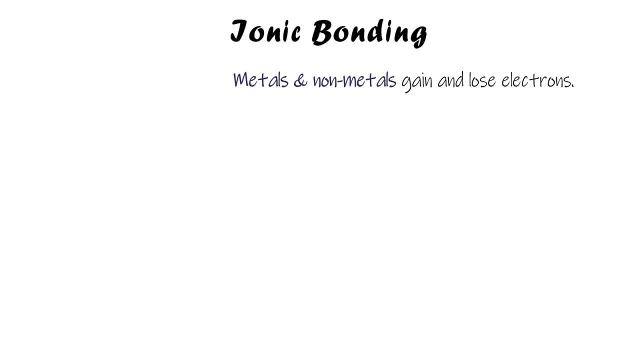 both metals and non-metals. It won't work unless you've got at least one of each- metals and non-metals- reacting together, And this time, instead of sharing the covalent bond, you're going to have just two of those. So you've got. 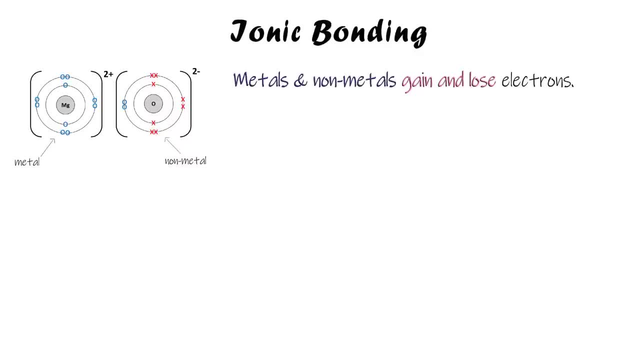 one and the other, And the third one, which has three electrons and four electrons. your side is going to be non-metal, So you work with two elements. We know that we can find an ion and a non-metal when we combine the two and determine theでは with an ion. Now 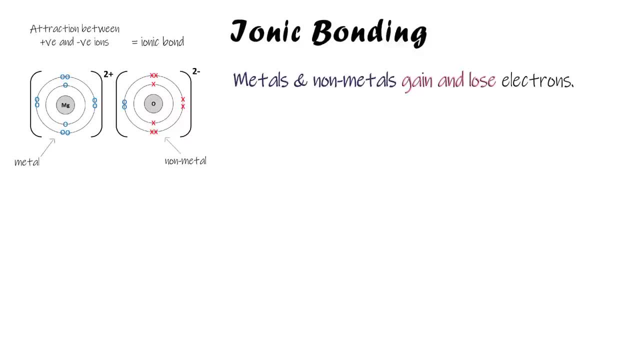 that phrase works like so. So if, in this case, if we're just adding atoms of方面 diamond, there'll be an attraction between them and that attraction is our ionic bond. so the definition of an ionic bond is a strong electrostatic attraction. that is a really, really important. 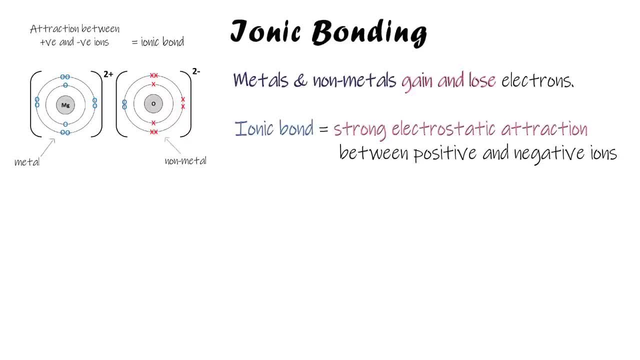 key phrase. that just means attraction between positive and negative, and in this case it's between positive ions and negative ions. so we have our positive and negative ions arranged like this in this big crystal structure- and this would happen thousands and thousands of times over with thousands of atoms- and there's that attraction between positive and negative ions. 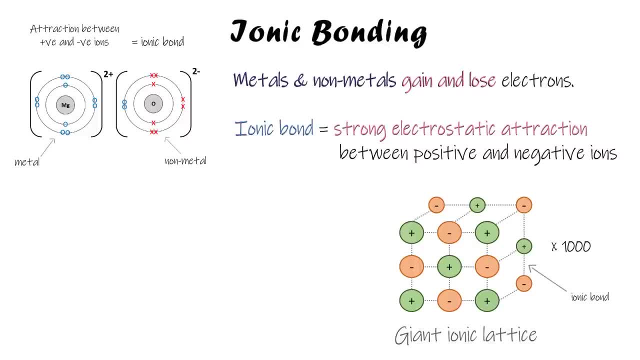 that is your ionic bond, that strong electrostatic attraction. this structure where you've got thousands of ions repeating in that structure is called a giant ionic lattice. some examples of ionic compounds will be calcium chloride, magnesium oxide and aluminium bromide. so you can see in each of these chemical. 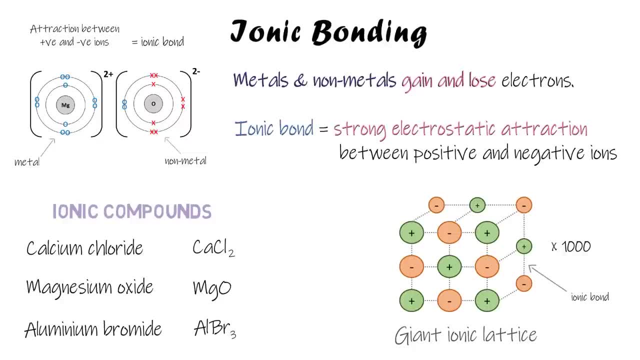 parameters. if you look at the formulas, we've got a metal and a non-metal. so calcium is a metal, whereas chlorine is a non-metal. in magnesium oxide, magnesium is a metal and oxygen is a non-metal. and in aluminium bromide, aluminium is a metal and bromine is a non-metal. so you can see in. 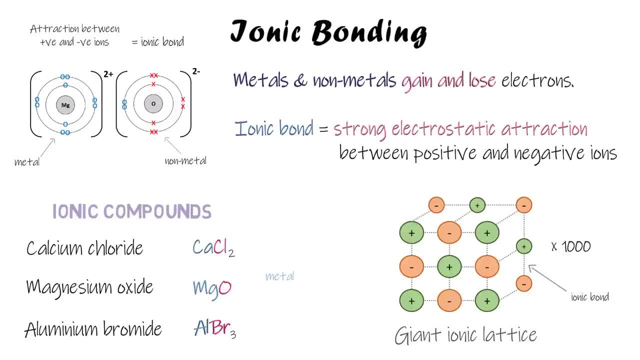 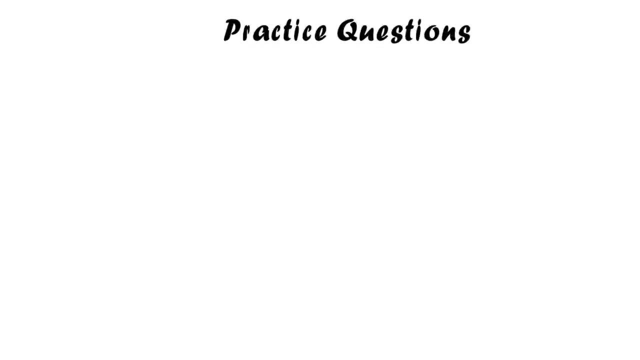 each case we've got both a metal and a non-metal element present, at least one of each. you could have each. it will not be ionic bonding unless you've got both a metal and a non-metal present. here's some practice questions about ionic bonding this time. so number one: what is an? 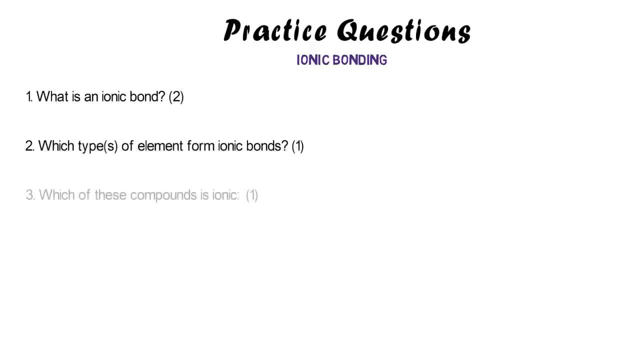 ionic bond, and note this, one's a two mark. question number two: which types of elements form ionic bonds? number three: which of these compounds are ionic? there's just one. in this case we've got sodium chloride, iron, diamond sulfate outside, or oxygen. pause the video and 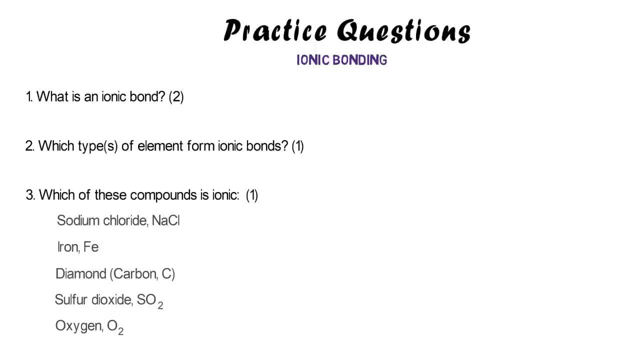 have a go. so the definition of an ionic bond is that it is a strong electrostatic attraction. electrostatic is about positives and negatives. this time it's between positive ions and negative ions. the positive and negative ions are attracted to each other. that's the dotted lines in this diagram. those are your ionic bonds. 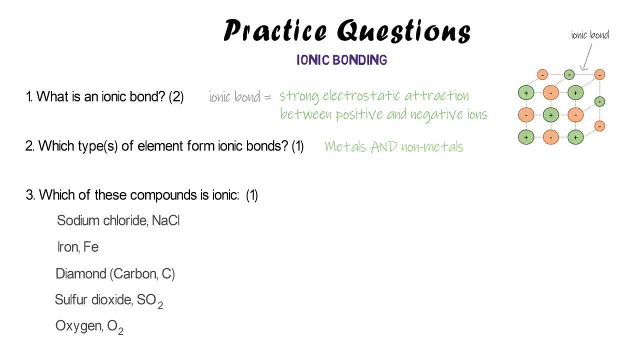 the types of elements that form ionic bonds are metals and non-metals. you can only get an ionic bond forming if you have a metal and a non-metal reacting together, and of those compounds and elements, sodium chloride is the only one that has a metal. 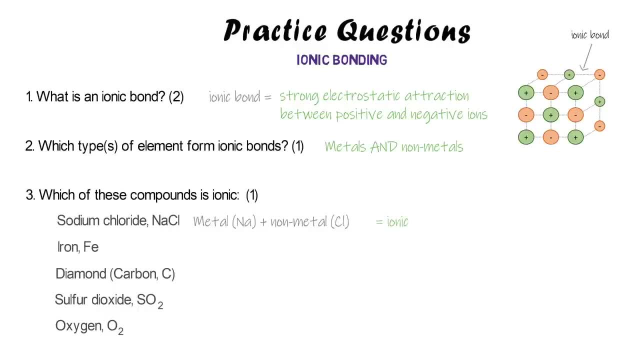 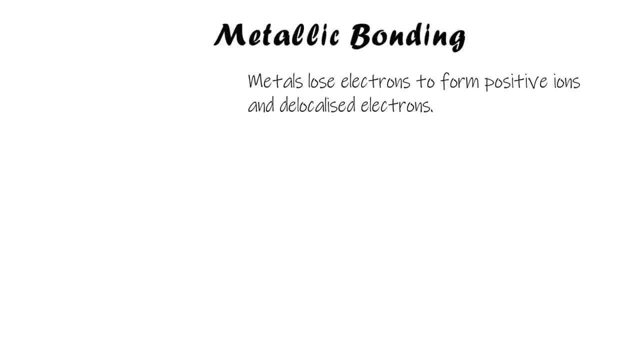 and a non-metal present sodium and chlorine, so that means that must be the only one that's ionic. the last type is metallic bonding, and this happens obviously only within metals, so it happens inside a sample of a metal or between metals. the metal atoms lose electrons. 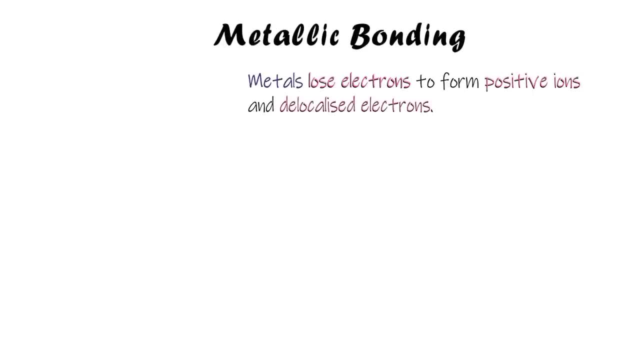 out of their outer shell and that makes them form positive ions. the electrons they lose become delocalized, which means they're no longer attached to any one ion and they kind of float around in this sea of delocalized electrons. we've got positive ions and then a sea of delocalized 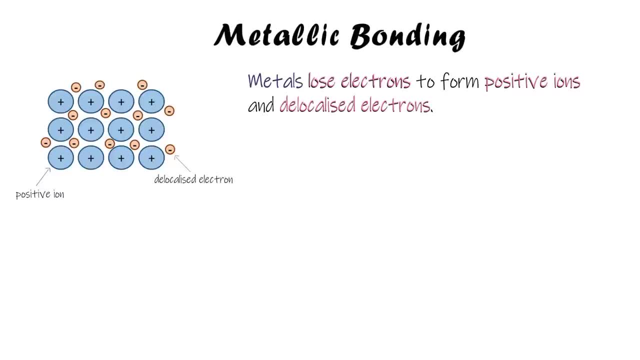 electrons float around in this sea of delocalized electrons, which is a non-metallic bond. so that's a. because the ions are positive and the electrons are negative, there's going to be an attraction between them, just like with ionic bonding: they're going to be attracted to each other. 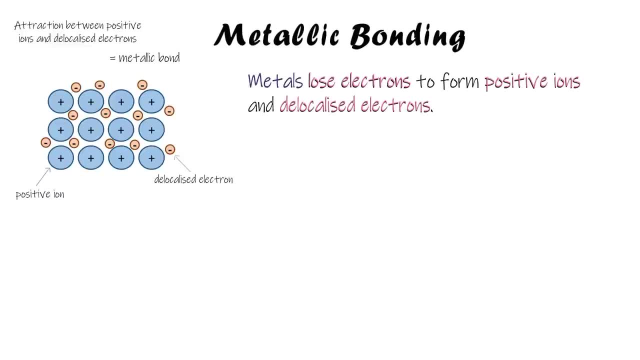 and this attraction between the ions and the electrons is the metallic bond. so the definition of a metallic bond is a strong electrostatic attraction. so it's the same key phrases with ionic bonding, but this time, instead of between positive ions and negative ions, it's going to 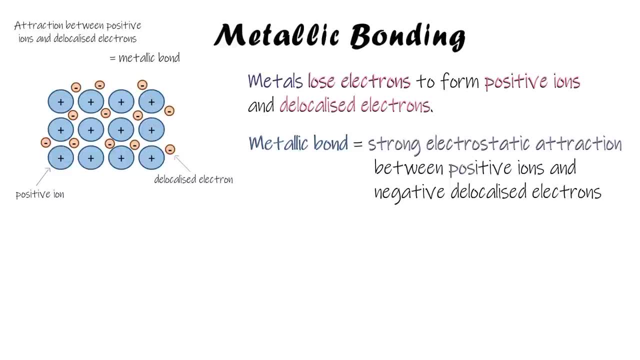 be an attraction between the positive ions and those negative delocalized electrons, and that attraction holds the metal together and it helps it keep its structure. the positive and negative are attracted to each other and that holds the metal together. this is what this giant metallic structure would look like. so again, in this case, just like ionic bonding, you've got many thousands. 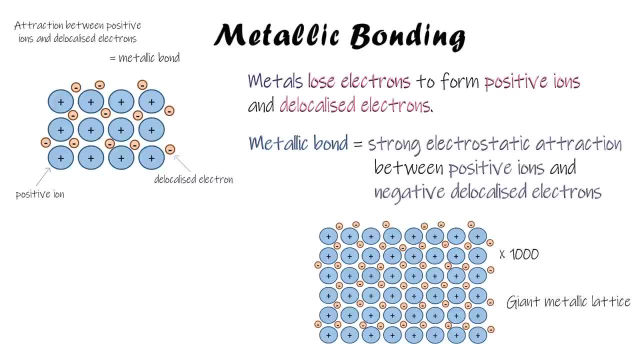 of atoms joined together in rows, forming this giant metallic lattice being held together by the ionic bond. and this is what this giant metallic structure would look like. so, again in this case, just like ionic bonding, you've got many thousands of atoms joined together by that attraction between the ions and the electrons. 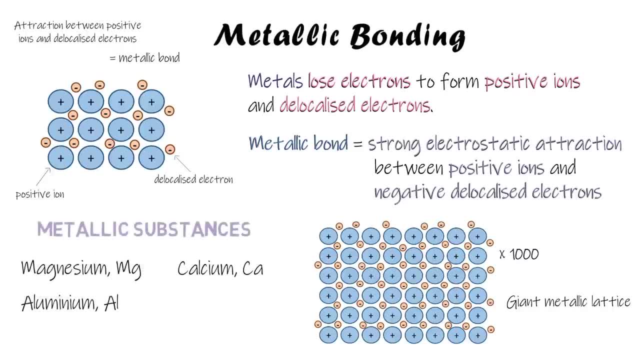 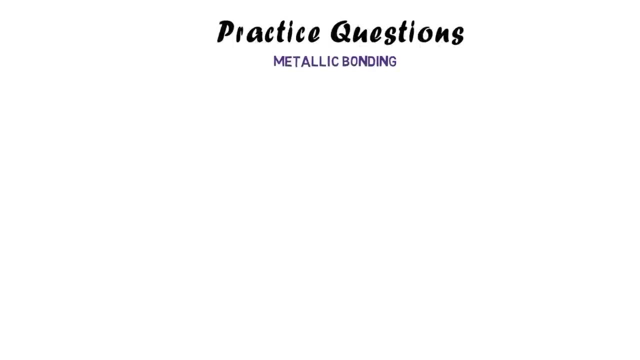 so examples of metallic substances would be magnesium, calcium, aluminium, copper, sodium and iron. so things that are on the left of the periodic table and some final practice questions for metallic bonding. number one: what is a metallic bond? number two: which types of element form metallic bonds and what is a metallic bond? 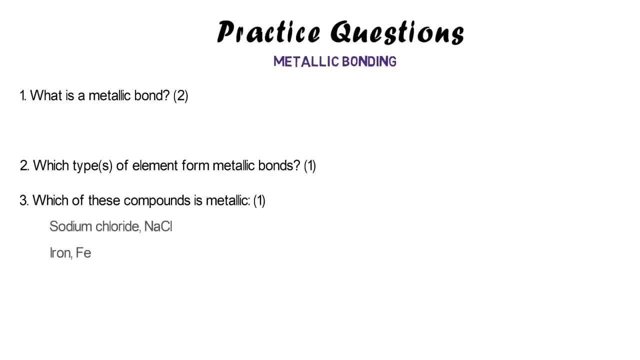 number three. which are these compounds are called metallic bonds? and number three, which of these compounds is metallic? pause the video and give these questions ago. the definition of a metallic bond is that strong electrostatic attraction that gets you first mark. and this time it is between the positive ions and not negative ions, it's the negative and the positive ions. 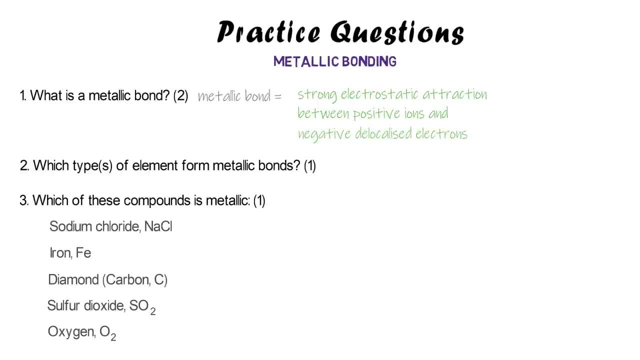 the negative delocalized electrons. so that's how it's slightly different to ionic bonding. so instead of between positive and negative ions, it's between positive ions and negative electrons. the attraction between them is your, is your metallic bond. it only happens within metals, never between non-metals. and of all those compounds, iron,